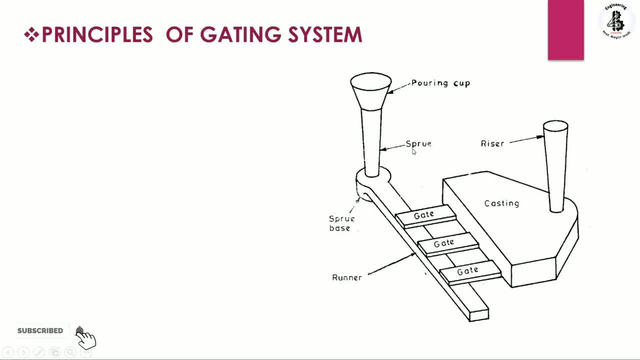 that will be connected with the sprue. So basically, sprue it will be a vertical passage for a molten form of the metals So it will be collecting into the sprue base. So at the end of the sprue it will be our sprue base. So all the molten form of the 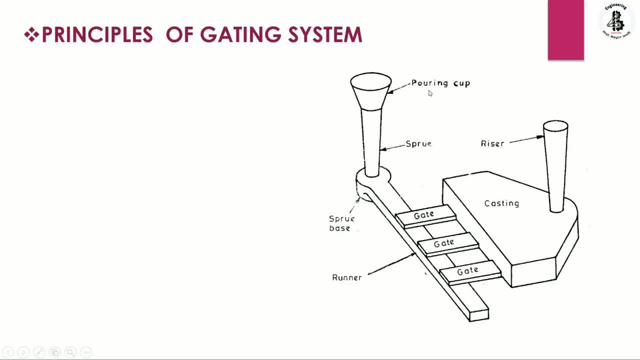 metal. first it will be collecting into the pouring cup and, with the help of sprue, once again it will be collected at the sprue base and sprue base that will be connected with a runner. So, as from my shape and size, this runner is being designed and runner. it will be connected with the different 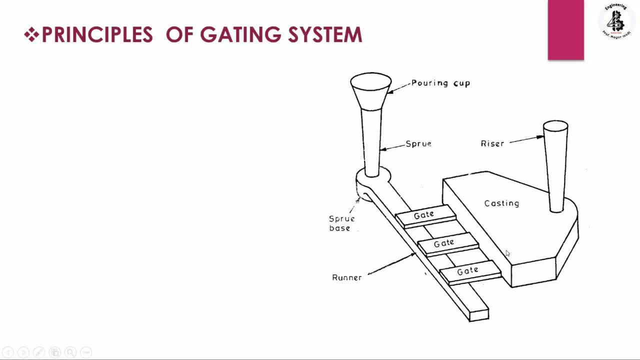 getting systems. So here that will be. the size is larger, So the three different getting systems is being arranged for: easily pouring the molten form of the metals with the help of pouring cup, sprue, sprue, base runner, and getting systems towards the 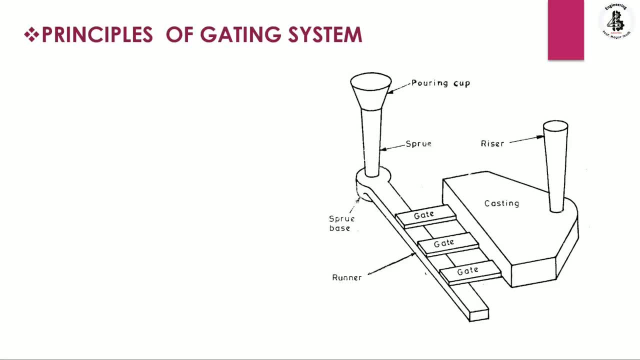 castings or you can say cavity. So at the end of the castings there will be a riser. So basically the function of the risers. if you find the molten form of the metals after the pouring from the pouring cup, So that will be gives the 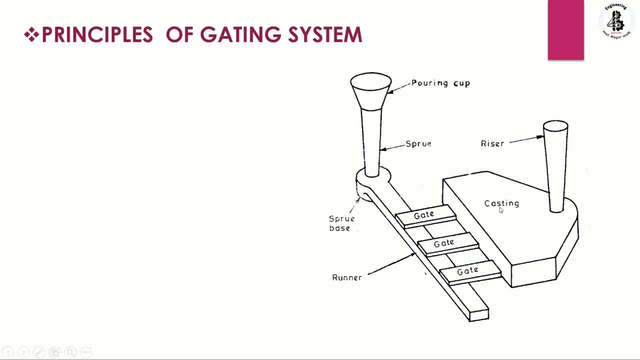 100% ensurement regarding to the filling of the castings, or you can say 100% filling of the mold cavity. Second thing: into the casting process, the molten form of the metals. it will be solidified and during the metal is being solidified it get shrink. So due to that shrinkage, that additional 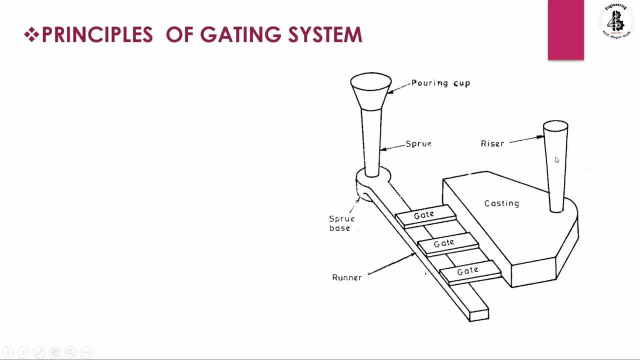 matters it will be providing into from the risers. So that will be the second functions of the risers and that risers it will be also help for escaping the air is being present into the mold cavity, or you can say castings, before the molten metal is being entering. So just you can see the term getting. 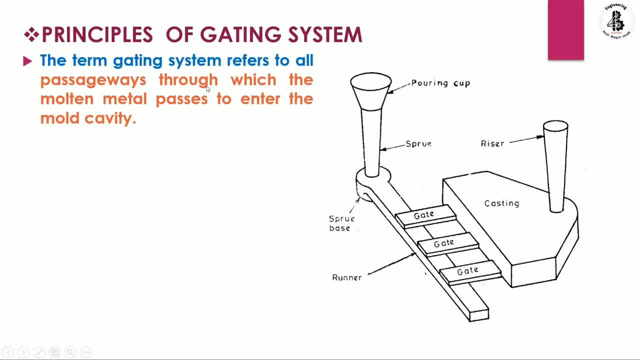 systems refers to all the passageways through which the molten metal passes to enter the mold cavity, So that channel, or you can say sprue, runner and riser arrangement. so that will be basically the principles of the getting systems. So the getting systems is composed of pouring cups. 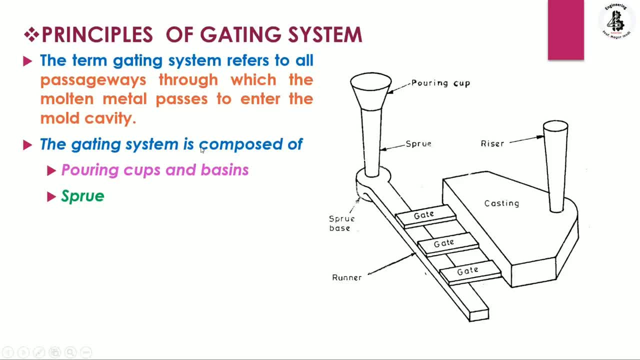 and basins. secondly sprue, then runner, then different getting systems as per the my requirements risers. So just you can see this is our pouring cup, or you can say pouring basin. then, second important part, it will be the sprue, it will be connected with. 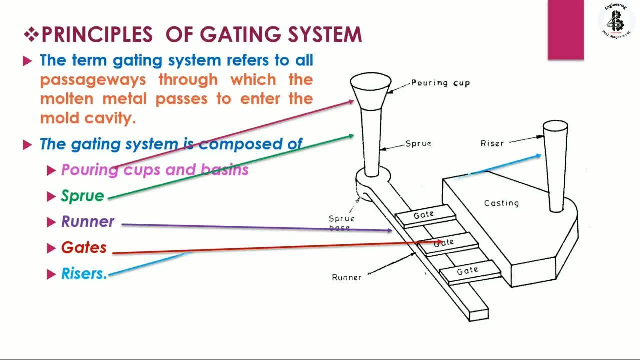 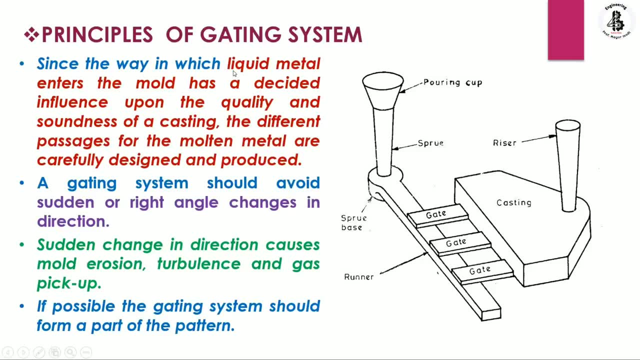 the runner, then getting systems and finally it will be a riser. Then just you can see, since the way in which the liquid metal enters the mold has a decided influence upon the quality as well as the soundness of the castings. So the different 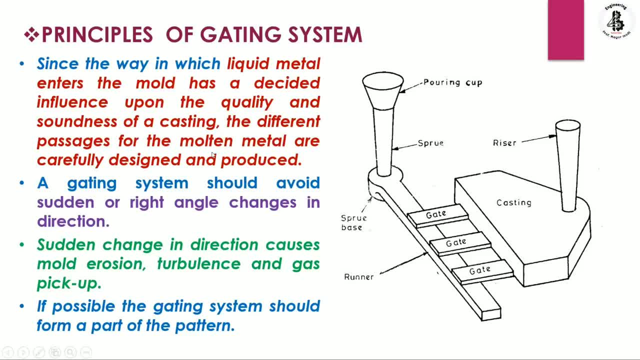 passages for the molten metals are carefully designed and it would be produced So into the getting ratio designs what you take care about it, The cross sectional area of the sprue runner and riser, then, and then you should controlling the flow of the molten form of the metals. So basically, a getting system should avoid sudden, or you can say: 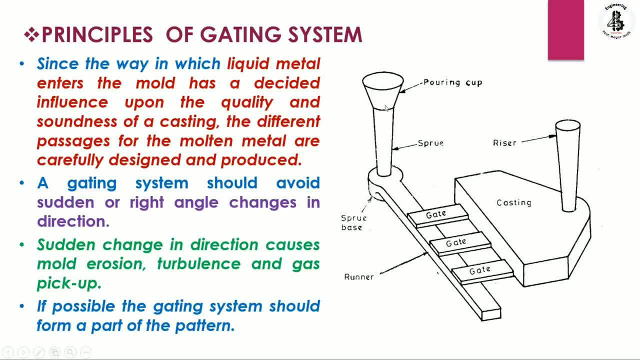 right angle changes into the directions. So just you can see here that will be the pouring cup and it will be connected with the sprue at the end of the sprue. just you can see once again. once again it will be collection of the molten form of the metal into the form of sprue base. 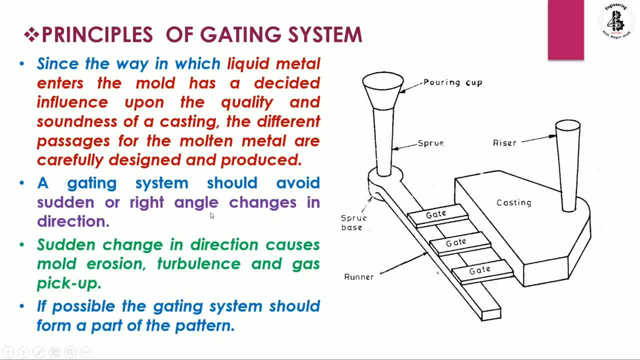 So that will be the avoiding the sudden- or you can say right angles- changes into the directions. Second things: the sudden changes in direction causes the mold, erosions, turbulence and gas pickups. So indirectly that will be reducing the characteristics of the getting systems as well as the casting products. 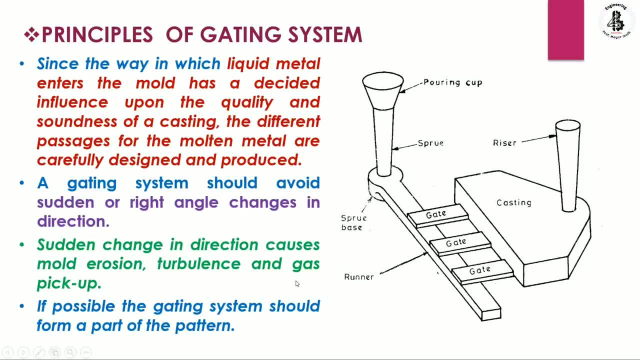 So if possible, the getting system should form a part of the pattern. So if pattern주이 So consider your INTERS amorous videos in our channel, the pattern he will be look like this kind of shapes. so that will being having better results, or can you will get some. 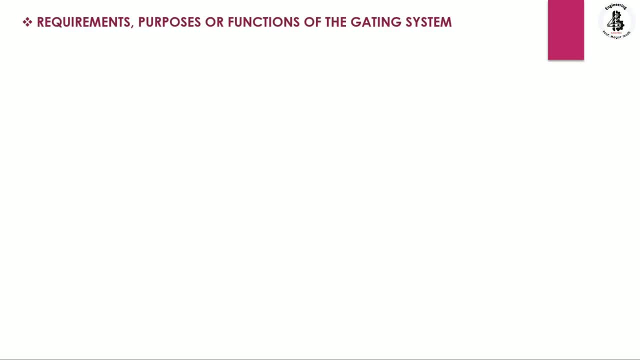 cost, Then the basic requirements purposes, or you can see different functions of the getting systems So that see a getting system should fill the mold cavity completely before the phrasings, So that insurance it will be given by the riserисor TransTPLAY.